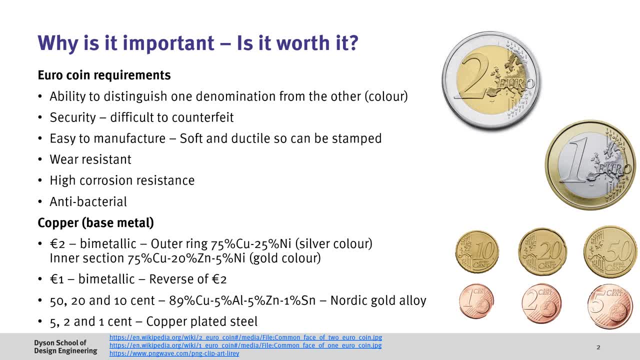 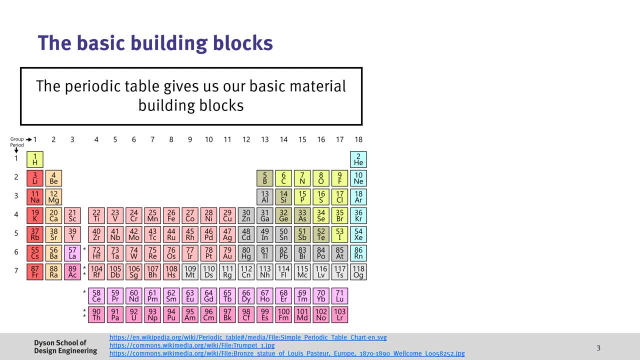 then people would just collect these and melt them down, which is obviously not what we want. Now, if we look at what options we have for material selection, the periodic table gives us our basic building blocks. This consists of over 100 elements, which might sound like a lot. 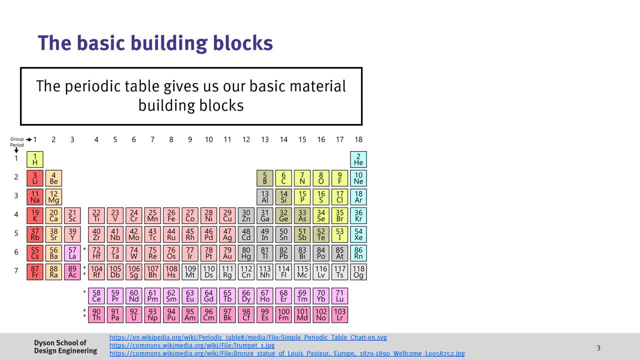 but many of these are either scarce or would be unsuitable in most material selection problems, thus limiting our options. However, if we mix elements together or alloy them, this allows us to augment the material properties and opens up many possibilities- The types of elements that we 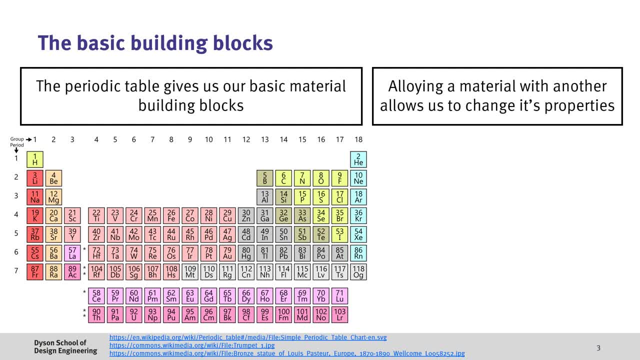 alloy together. their proportions and processing conditions have a huge impact on the eventual properties. Let's take, for example, bronze. This is an alloy of copper and tin and it's relatively hard and resists corrosion, which makes it ideal for making statues. However, if we change стан for 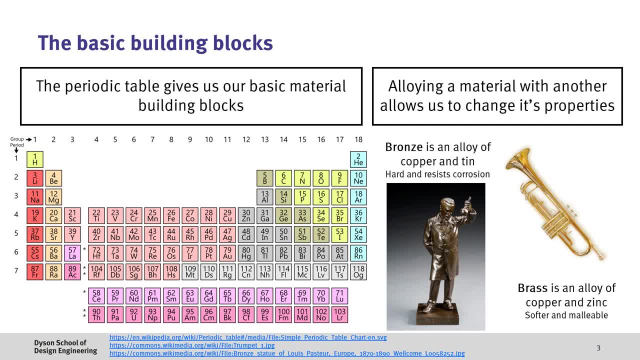 zinc. we can then make brass, which is softer and more valuable, making it suitable for manufacturing musical instruments. Therefore, you can see that alloying materials have better emllers, As you can lekker bet Jacobs посмотреть. Instead of restoring compressed elements, it is more effective infaturing whole pieces. 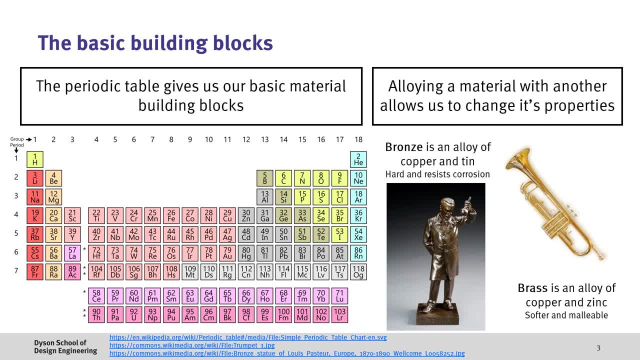 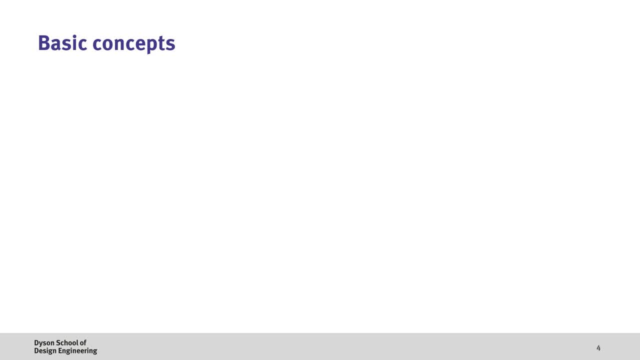 thinner pieces. houses from a long distance like pay it off, but allow the metals to osmar as naturally as possible. alloying materials has a strong influence on its material properties, and phase diagrams can help us understand what's happening. so now let's look at a few basic concepts which we'll be discussing. 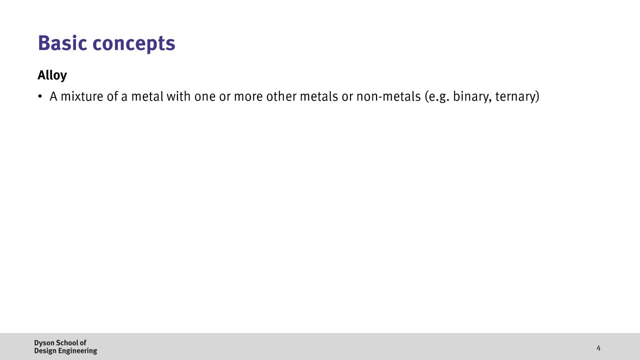 in more detail throughout the video. firstly, the term alloy refers to a mixture of a metal with one or more other metals or non-metals. we term this binary when we have two elements and ternary when we have three, and so on. when talking about a component, we're referring to an element in the 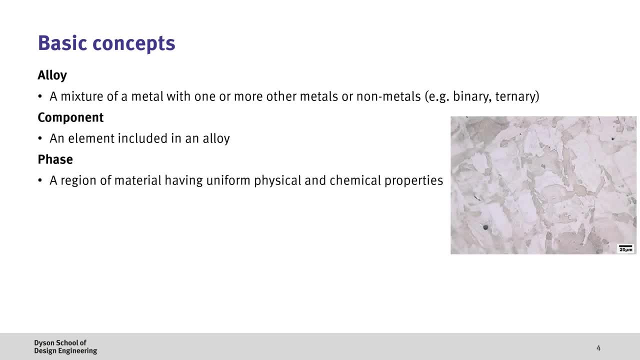 alloy, a phase is a region of a material which has uniform physical and chemical properties. this is an important concept that we'll come back to later on. in the image that you see here, this is an optical micrograph of steel, which is an alloy of iron and carbon. the different 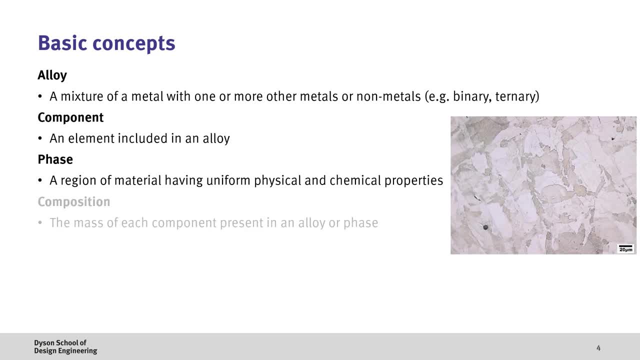 colored grains. you see, here are different phases. the composition of a phase is the mass of each component in the alloy or phase. the constitution is the sum of the phases, the mass of each phase and the composition. and finally, the phase diagram is the equilibrium constitution of all of the combinations of temperature and composition for that particular alloy. 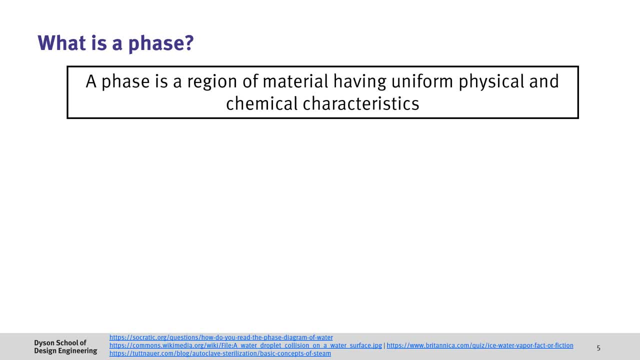 now, given that this video is about phase diagrams, it's worth discussing in a bit more detail about what a phase is. earlier, we defined as a region of a material which has uniform physical and chemical characteristics. but let's have a look at an example to help us visualize this. The plot you see here is the phase diagram. 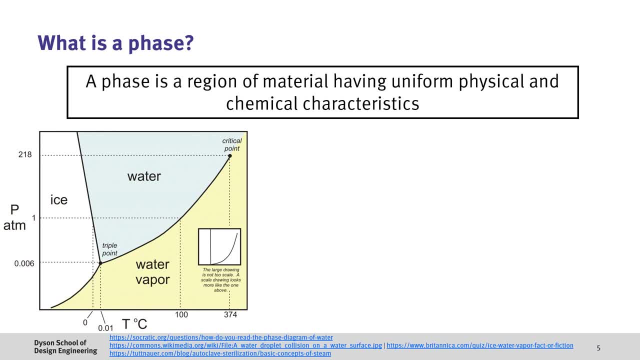 for H2O, where the x-axis is temperature and the y-axis is pressure. Now we know, at room temperature and atmospheric pressure, H2O exists as a liquid state known as water. As we decrease the temperature below zero degrees C, the H2O undergoes a phase transformation from a liquid to a solid. 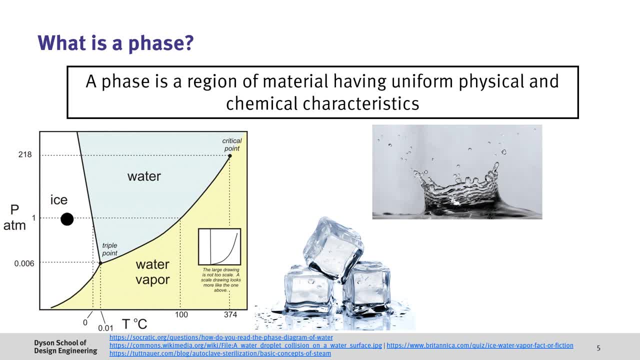 we know as ice. Clearly, the physical properties of water are very different to ice. If we then increase the temperature to above 100 degrees C, the ice transitions to a liquid and then to a gaseous steam. Again, steam has very different physical properties to ice and water, but it has 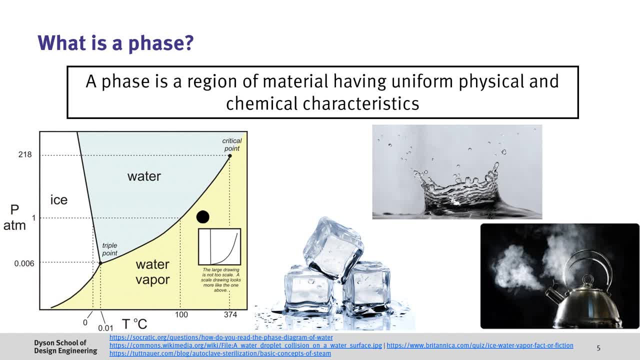 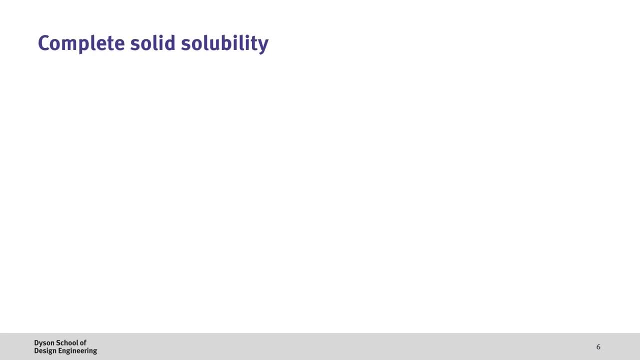 the same composition. So what this tells us is that temperature is very important When describing the physical properties of a material. Now, when we start to mix different elements together, a number of different things can happen. If the two elements are similar to each other, they can form what we call a solid solution. A solid solution is a single phase region. 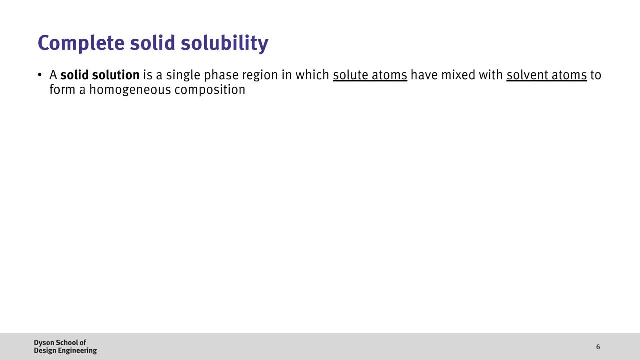 in which the solute atoms have mixed with the solvent atoms to form a homogeneous composition. The term solute atoms refers to the elements in the smaller proportion, and the solvent atoms refer to the element in the larger proportion, If the two elements are very similar to each other. 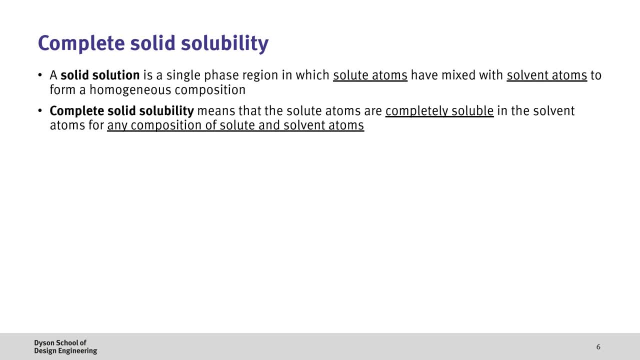 they can have complete solid solubility, which means the solute atoms are completely soluble in the solvent atoms. for any composition of the solute and solvent atoms, A second phase therefore does not form. In order to visualize this principle, let's take the example. 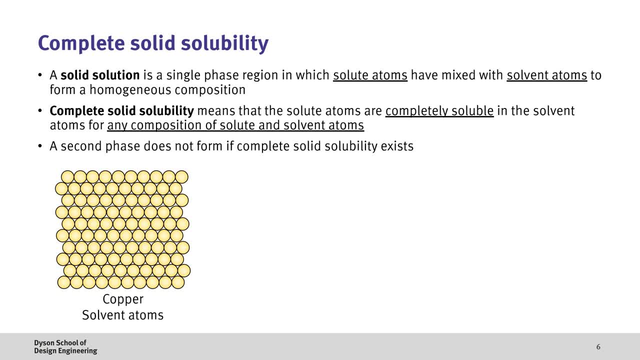 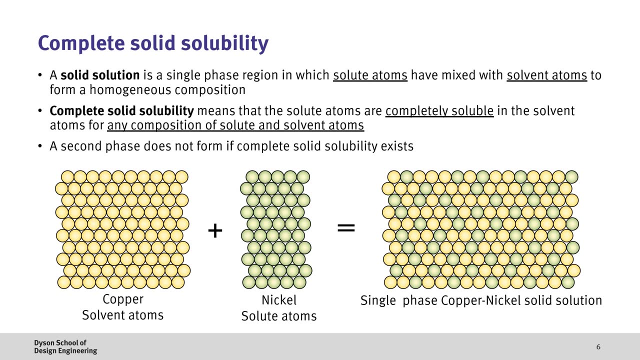 of a copper alloy. Here you can see a cartoon which represents the copper, which is the solvent atom in this case. We then want to alloy this with nickel, which is the solute in this case, since there's a smaller proportion of this element In the case of copper and nickel. they 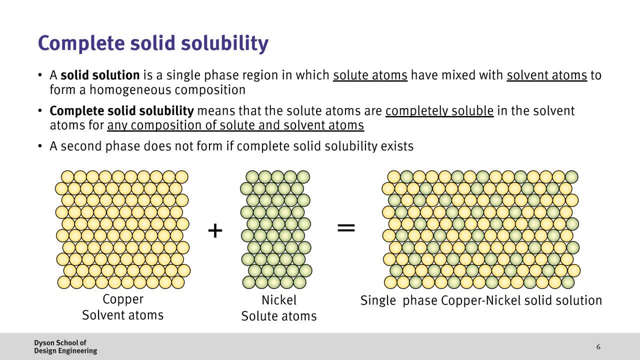 have complete solid solubility and therefore for any amount of copper or nickel they'll form a homogeneous phase with uniform physical and chemical properties, as shown in the diagram. If we dive a bit deeper into alloys which have complete solid solubility, we can start to see the 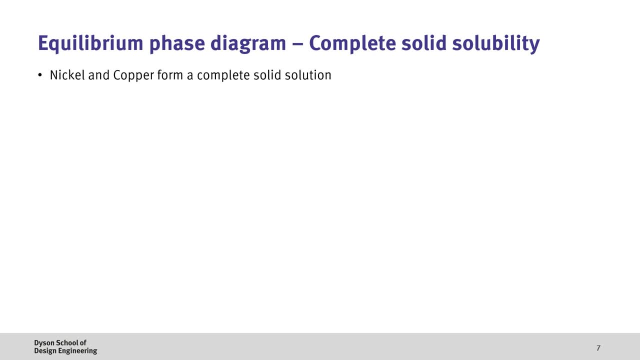 utility of the phase diagram. So let's look again at a nickel copper alloy example which exhibits complete solid solubility. From our earlier example with H2O we know that temperature is a key metric for determining the phase and physical properties of a material. In the case of nickel, the melting 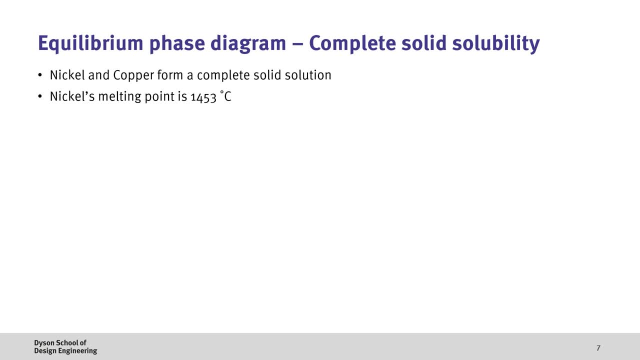 point is 1453 degrees C. Copper, on the other hand, has a lower melting point of 1453 degrees C. Now, if we draw the equilibrium phase diagram for the copper and nickel alloy, it looks something like this: On the x-axis we have the composition in terms of weight percentage. 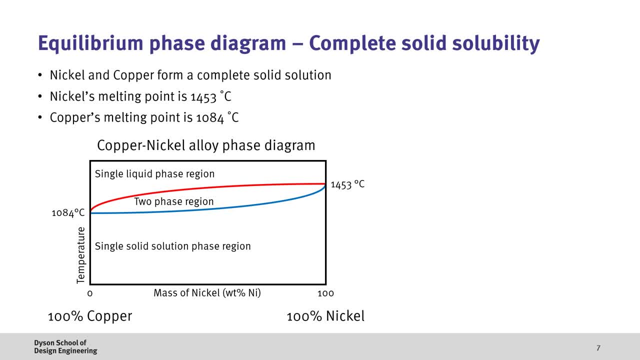 of nickel, and on the y-axis we have temperature. We can also see several lines which represent the phase boundaries between different regions. Here we've got three distinct regions: a single phase liquid region, a single phase solid solution region and a two phase region. 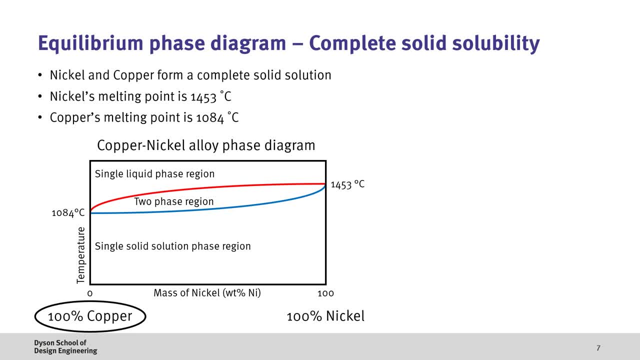 Given that this is a binary alloy of two metals, copper and nickel. when the weight percentage of nickel is zero, this means that we've got a hundred percent copper, and when we have a hundred percent nickel, we have zero percent copper. Now, if we assume we have an arbitrary composition of 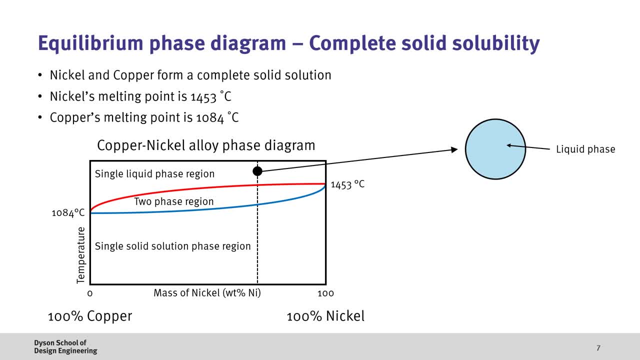 nickel and copper. where the temperature is above the melting point of nickel, we'll be in a single phase region where the structure will look very homogeneous. Given that we're using the term phase, it's useful to remind ourselves what that actually means. So a phase is defined as a region of a. 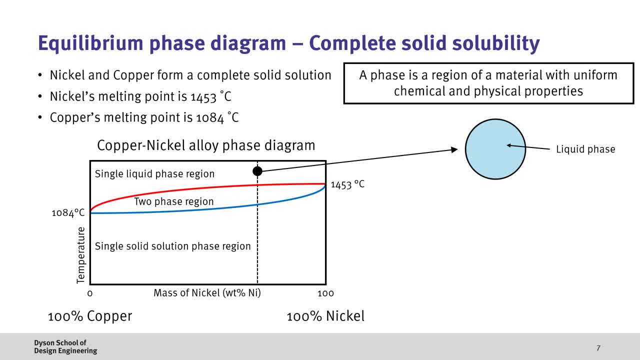 material with uniform chemical and physical properties. So at this temperature and composition everything will behave like a liquid. As we cool the alloy, the overall composition stays the same, but then a solid phase starts to precipitate out of the liquid. We can see that eventually all of the liquid becomes a solid, where the grains which initially 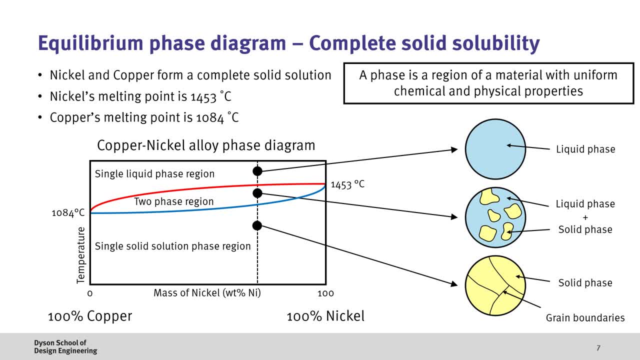 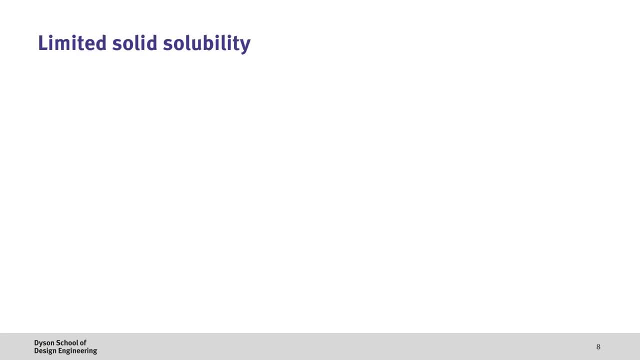 started to form, have grown and joined together. Where these grains join are what we call grain boundaries. So that was the situation where two metals have complete solid solubility. However, in many cases, where the two metals are considerably different from each other in terms of atomic size and charge, complete solid solubility isn't possible. Limited solid solubility: 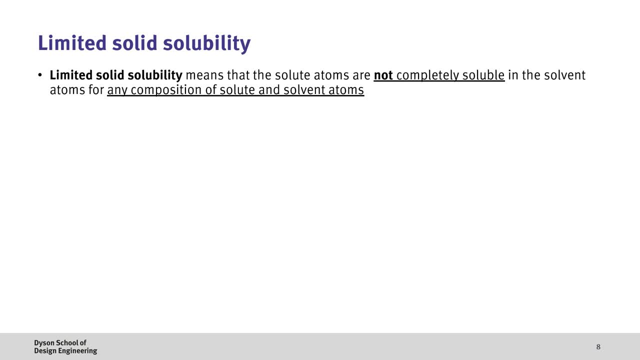 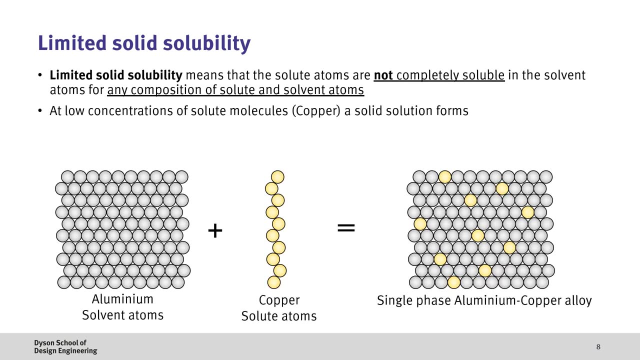 means the solute atoms aren't completely soluble in the solvent atoms for any composition, and therefore a second phase often forms. Now let's have a look at the example of aluminium and copper. These two elements don't have complete solid solubility, however at low. 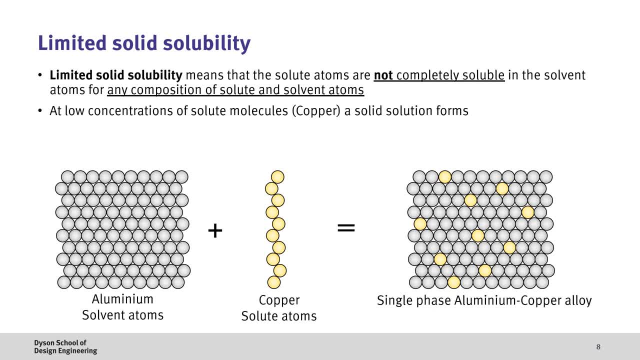 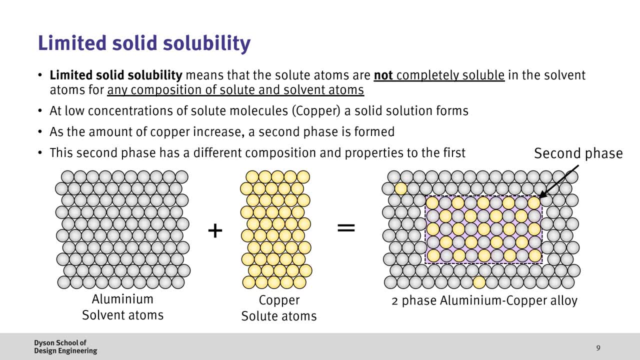 concentrations of solute atoms, a solid solution can still form, as shown in the diagram. However, as the concentration of solute atoms increases in a limited solid solubility system, a second phase can precipitate out, as this is more thermodynamically stable. Here you can see in: 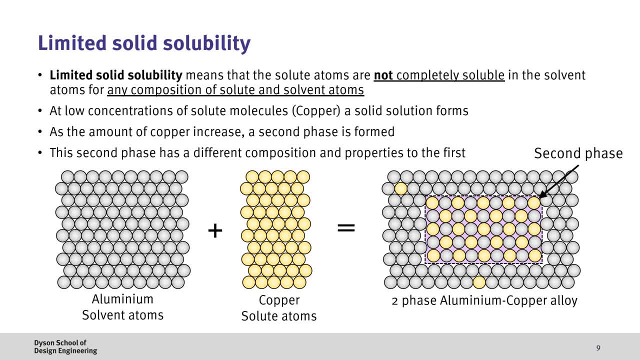 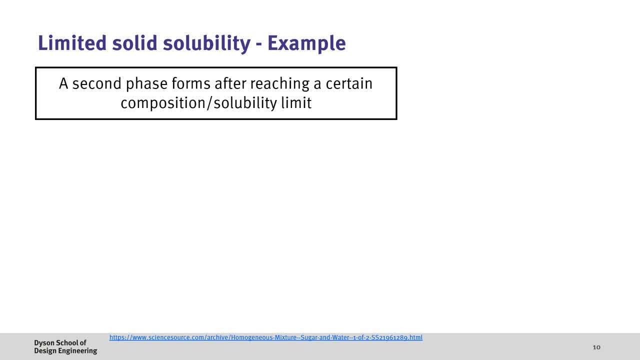 the diagram that, as we add more copper, a different phase has formed where the composition and structure has changed. Now this can seem a little bit abstract, so let's have a look at an example of a limited solid solubility system which you might come across in your everyday life. 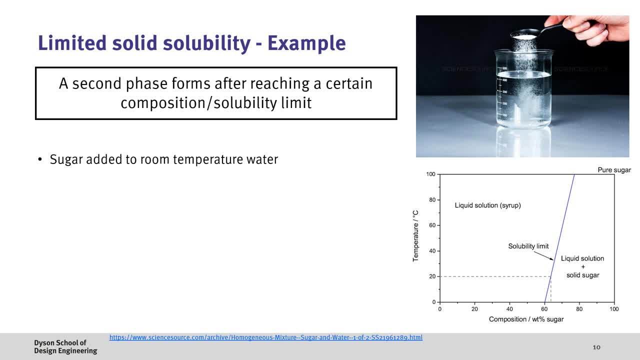 Here. let's take the example of adding sugar to water. The plot on the bottom shows the phase in the solution is the phase of sugar. The phase in the solution is a mixture of water and sugar. The x-axis is the weight percentage of sugar, where zero percent sugar is a hundred percent water. 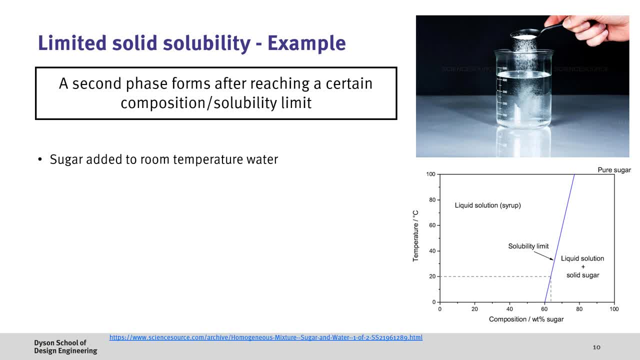 and vice versa. On the y-axis we have temperature and we can also see two regions, Initially at low concentrations of sugar. this dissolves completely to form a single phase syrup. However, as we add more and more sugar and pass the 65 percent solubility limit, the liquid can't. 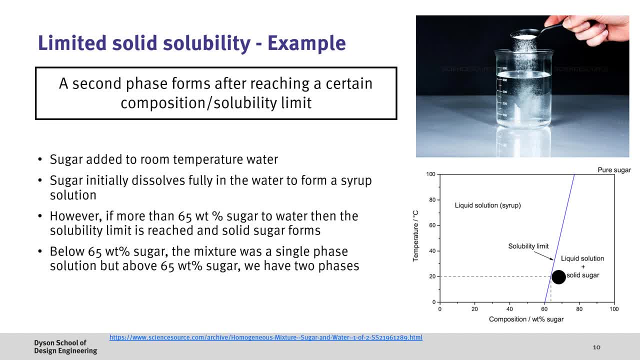 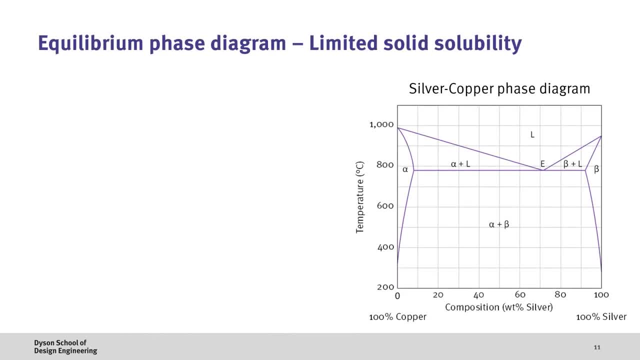 more sugar and solid sugar starts to precipitate out, leaving us with a two phase system of liquid syrup and solid sugar. Now, if we return back to our binary metal alloy system and look at silver- copper alloys, which have limited solid solubility, this is what the phase diagram looks like. This 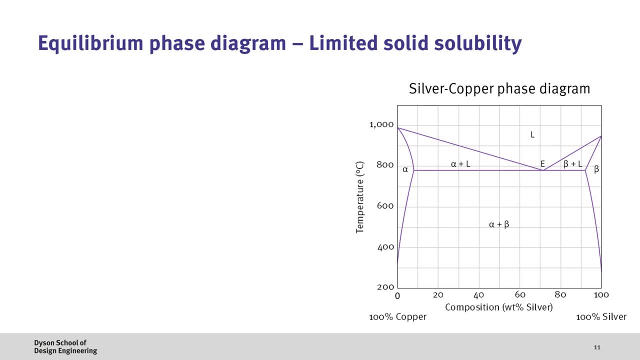 is obviously a little bit more complicated than the phase diagram for the complete solid solubility case, but we can break this down into more digestible parts. Here we have three single phase regions. Firstly, at low weight percentages of silver we form a solid solution with silver as the solute which we term alpha. Now the naming. 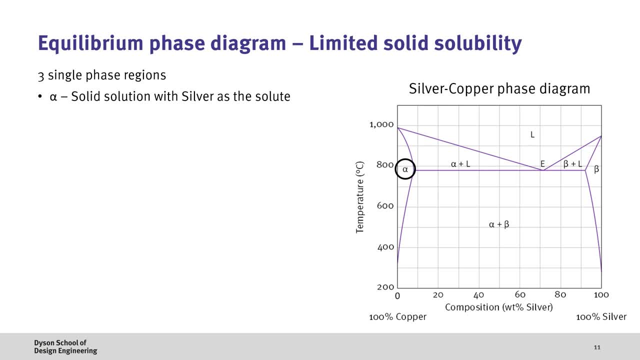 convention here is somewhat arbitrary, and in reality we could have called this anything else. Then, at high silver concentrations, we have another solid solution region, where copper is the solute, which we term the beta phase. At high temperatures we then have a pure liquid phase where everything has melted. Beyond these single phase regions, we also 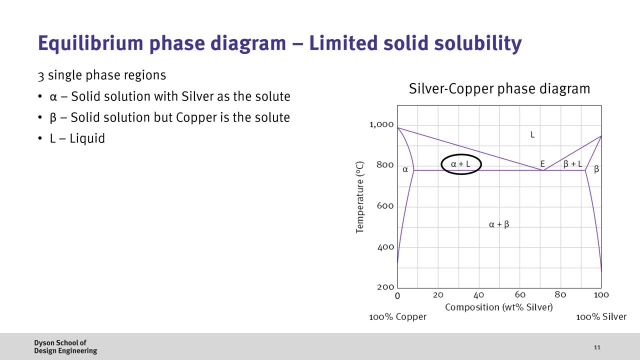 have three two phase regions where firstly, we have a two phase region of alpha and liquid, then we have a two phase region of beta and liquid and finally a two phase region consisting of solid alpha and solid beta. The lines on the phase diagram mark the boundaries between where these phases form and each of. 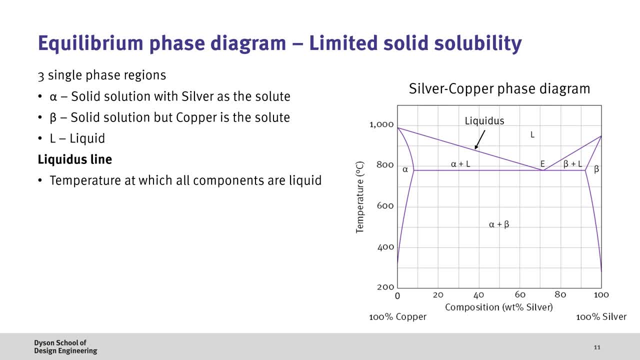 these has a different name. The liquidus line, for instance, represents the temperature and composition at which all components are liquid, The solidus line is the boundary beyond which no liquids form And the solvus line is the solid solubility limit between the alpha and. 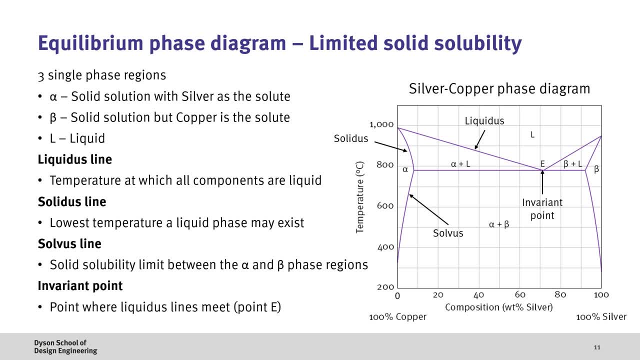 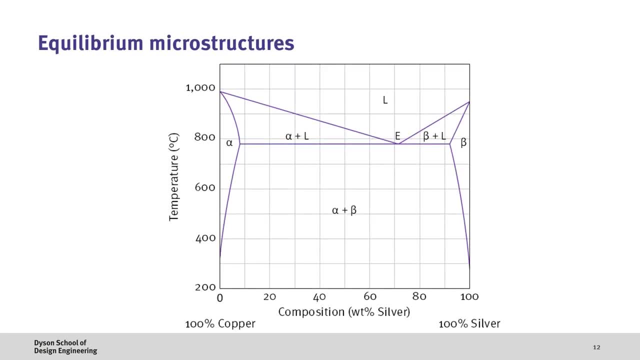 beta phase regions. We also have a region called the invariant point, where the liquidus lines meet, as shown by point E on the plot. Now, if we focus on this phase diagram and visualize the equilibrium microstructures which form, this will help us understand what's. 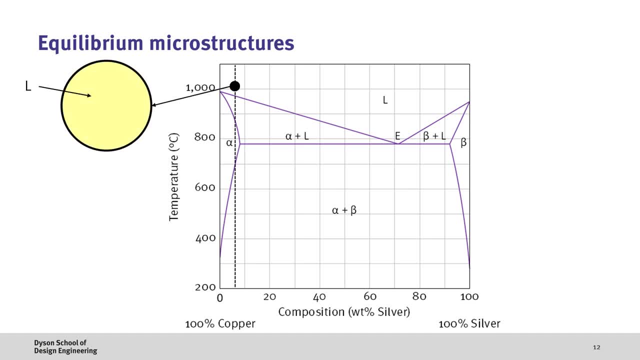 going on. If we select a low silver composition and start with a high temperature, we can see that we have a pure liquid phase. Then, as we decrease the temperature, we go through the liquidus line into the two phase alpha plus liquid region. Here the 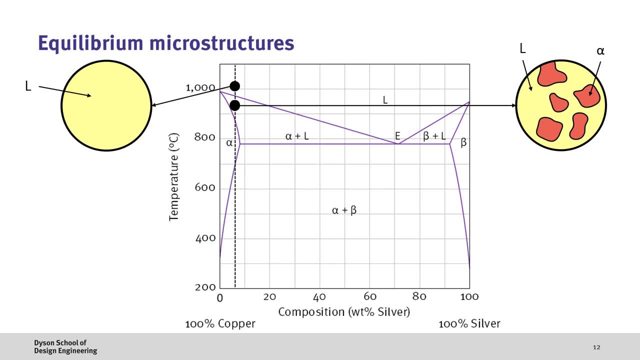 microstructure looks a bit like a soup with bits inside. Then, as we cool the material further, we pass through the solidus line, where all the remaining liquid has turned into solid alpha. Finally, if we continue to decrease the temperature, we pass through the solvus line. 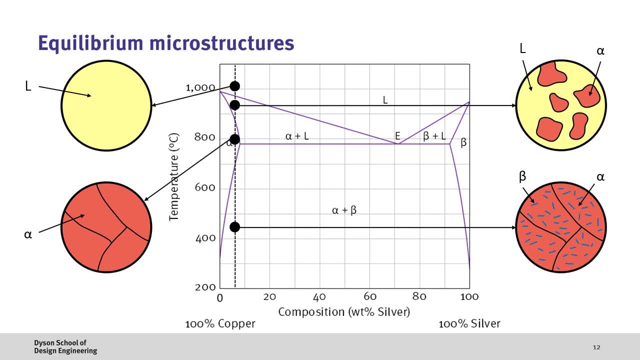 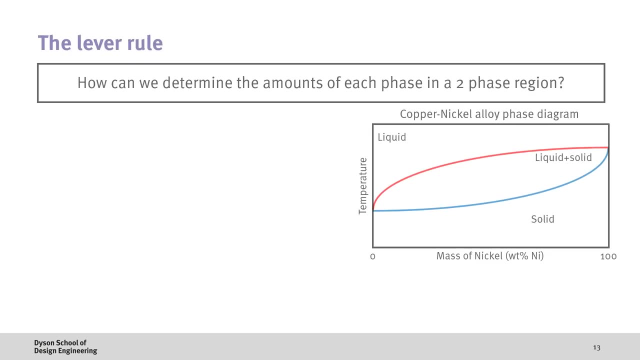 where the beta is no longer stable in the material and starts to precipitate out into a second phase. This type of microstructure with two phases can impact the mechanical properties of a material, since it can affect how easy it is for atoms to slide past each other. So that was useful to get. 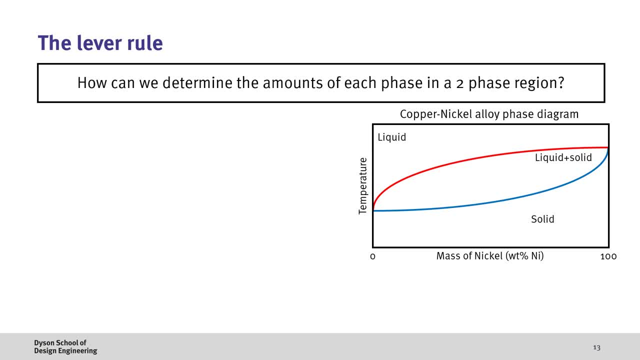 a qualitative view on what's going on in the material as we cool it. However, if we want to quantify the amounts of each phase in the two phase region, we have to take a slightly different approach. In this case, we can use something called the lever rule To run through this example. let's 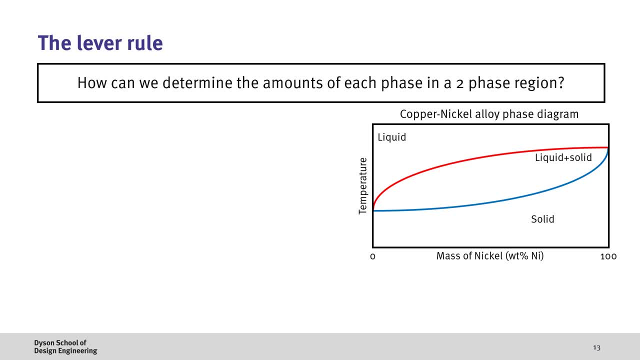 start again with a simple, complete, solid solubility system. First of all, we start by drawing a horizontal tie line at the temperature of interest in the two phase region. We then mark the overall alloy composition on this tie line, which we've arbitrarily put at 50% nickel If we want to. 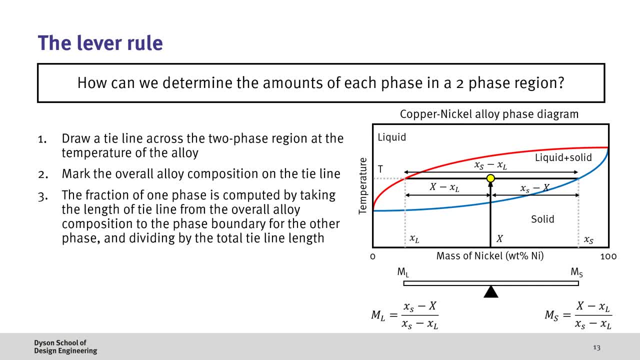 calculate the fraction of one phase. we do this by taking the length of the tie line from the overall alloy composition to the phase boundary of the entire alloy composition. Then we can calculate the total tie line length. This equation is given at the bottom for the generalized form describing: 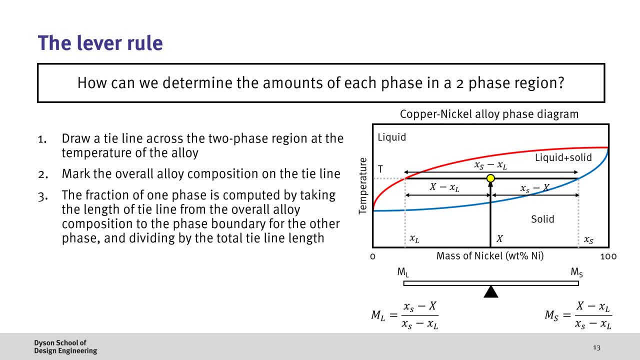 the mass of the liquid and the mass of the solid in this two phase region. If we now put in some numbers to help us visualize what this actually means, let's assume we have a 50% concentration of nickel, which means we have 50% copper in our alloy At this arbitrary temperature that we 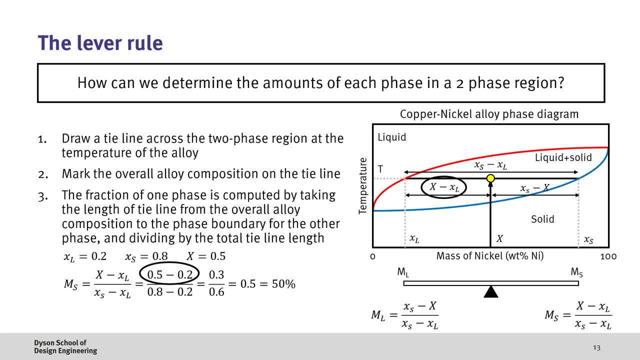 picked. the liquid solid phase boundaries occur at a rate of 20% and a rate of 80% nickel composition. If we then take the equations for the mass fraction of solid, we can see that the length of this tie line from the overall composition to that of the phase boundary is 0.5 minus 0.2, giving us our numerator. 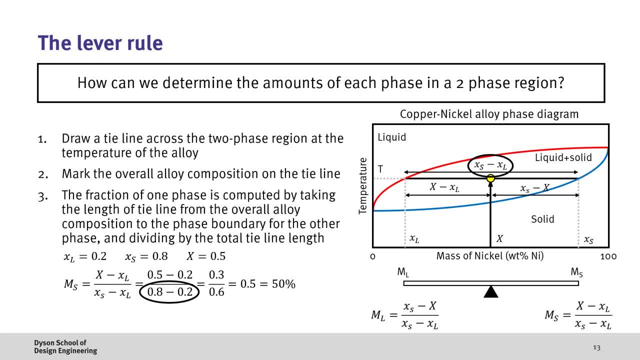 The length of this tie line is the composition of the solid phase boundary minus that of the liquid phase boundary. This acts as our denominator. If we then take the ratio of these two, we can see the mass fraction of the solid phase is 50%. We can then repeat this process for the liquid. 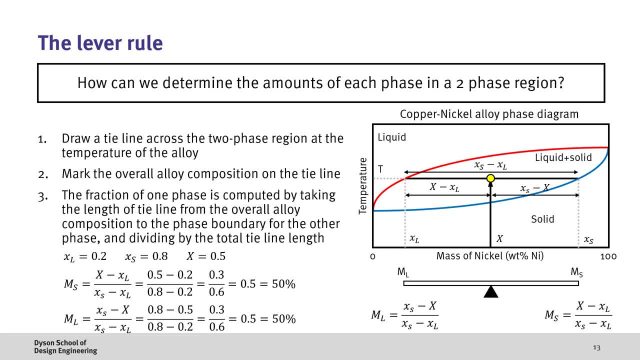 phase, which should also be 1 minus the solid mass fraction. Now let's say, for example, we increase the amount of nickel in our alloy to 80%. When we then put the numbers into our equation, we can see now that we have 100% solid and 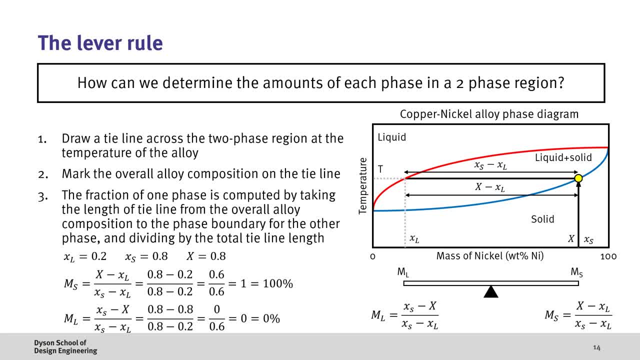 therefore 0% liquid. This makes sense, since we are now at the solidus line, where the entire alloy should be in the solid phase. Conversely, if we reduce the amount of nickel to 20%, we can see that the mass fraction of solid becomes 0 and therefore we have 100% liquid. This again makes sense, since we are 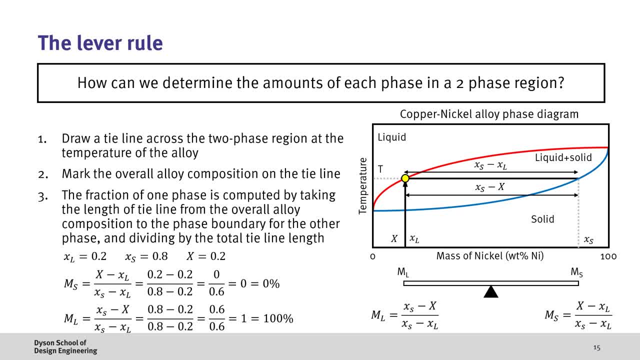 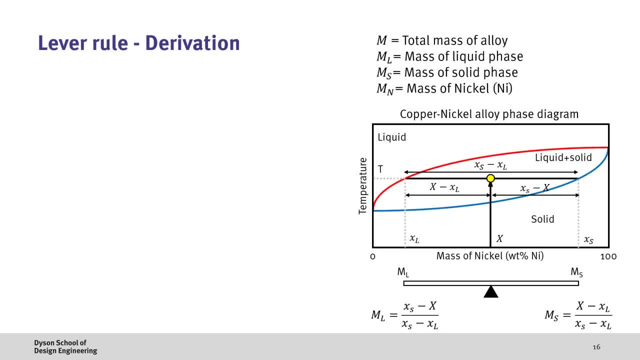 now at the liquidus line composition and highlights another important factor: that alloying metals allows us to control the melting point of the alloy. So hopefully that example of the lever rule helps you understand how to use the alloy to control the melting point of the alloy. 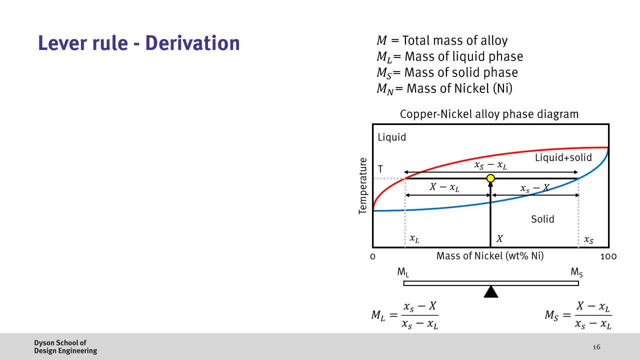 However, it's also useful to know how this is derived, so that we don't just take it at phase value. Now, to do this, we firstly take a mass balance of our two-phase alloy, which consists of a solid phase and a liquid phase. Since there's only two phases here, the sum of the two must 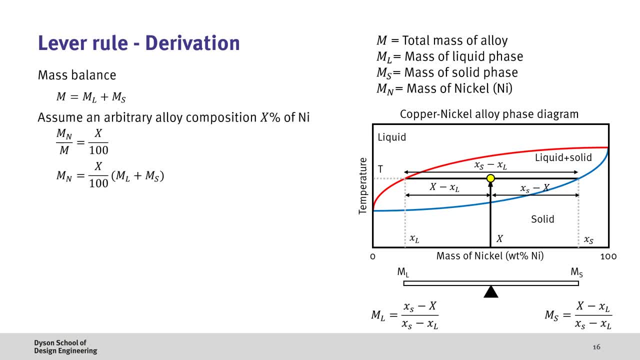 equal the total mass of the alloy. Next, if we assume an arbitrary alloy composition of x% nickel, we can say that the mass of nickel over the mass of the alloy gives us our mass fraction of nickel. If we rearrange this equation to: 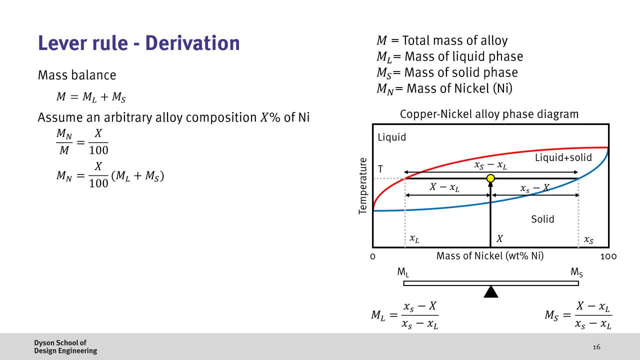 make the mass of nickel the subject and then substitute the equation in for total mass, we get a description of the total mass of nickel in the system. Now, if we create an independent mass balance for nickel, what we can say is that the total mass of nickel can be described as the mass fraction of nickel in the liquid plus the. 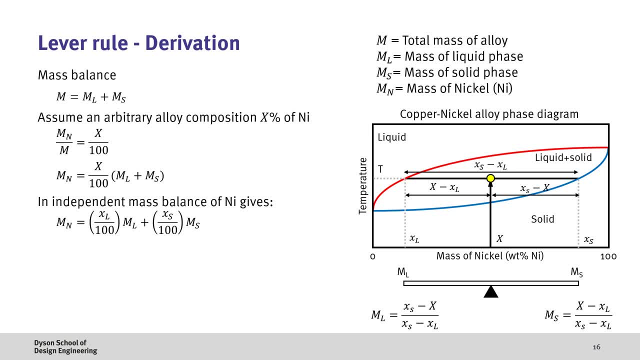 mass fraction of nickel in the solid, since these are the only two places where it could. so It's important to remember that nickel generally exists in both the solid and liquid phase. We now have two independent equations which describe the mass of the liquid, and if we 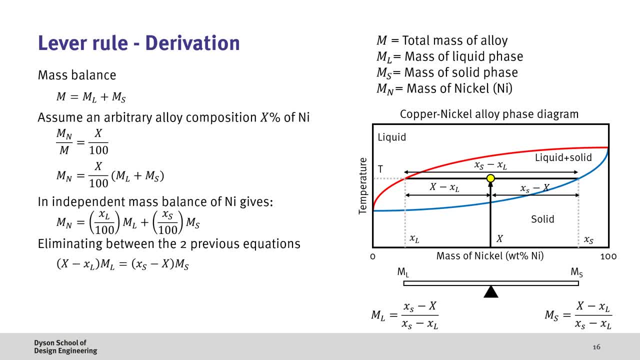 equate the two together and rearrange them slightly, we come to this equation. Finally, if we say that in the two-phase region the mass of liquid and the mass of solid equals one, we can then solve these equations of clearance for the mass fraction of liquid. 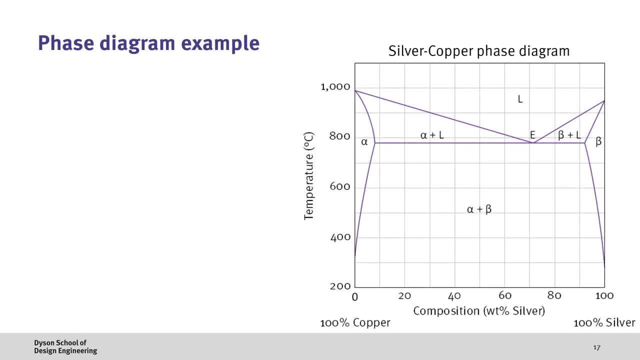 and solid. So now that we've done an example of how to use the lever rule for a complete solid solubility system and also understood where this comes from, let's look at a final example where we apply this to a limited solid solubility system, such as silver and copper. 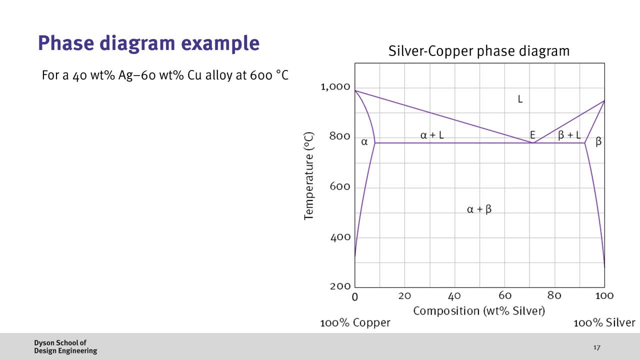 Let's say, for example, we have an alloy consisting of 40 weight percent silver and 60 weight percent copper at 600 degrees. Now the first question might be: what are the phases that are present at this temperature and composition? This is relatively straightforward, as we find the composition and temperature that we've 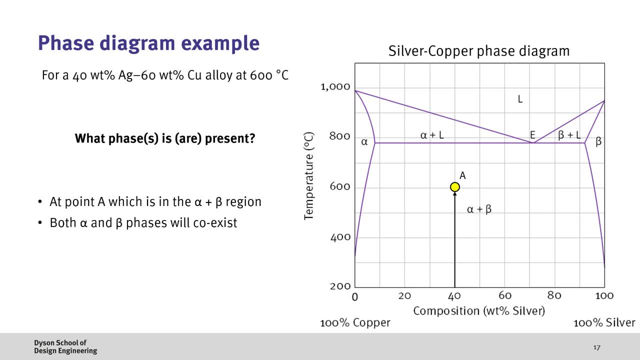 just mentioned, and then look at what region we're in in the phase diagram. In this case we can see that this is in the solid alpha plus beta two phase region. Now, whilst we know at 40 weight percent silver and 600 degrees we have two phases, what we 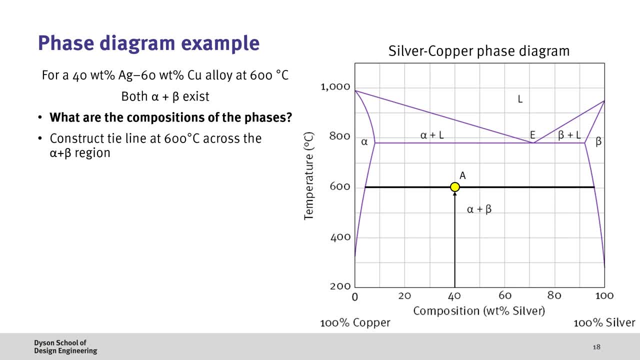 don't know is what their composition is. To answer this we can use the lever rule. First we draw a tie line at 600 degrees between the alpha and beta regions. Then if we read the composition of alpha at the solvus line, we can see that we have a. 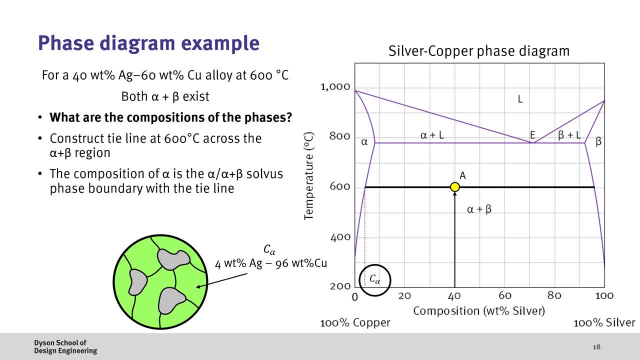 composition of 4% silver and therefore 96% copper. Since this is the point where we only have alpha, we can say that this is the composition of alpha. We can then repeat this process. Here. we can see that beta has a composition of 97% silver and therefore 3% copper. 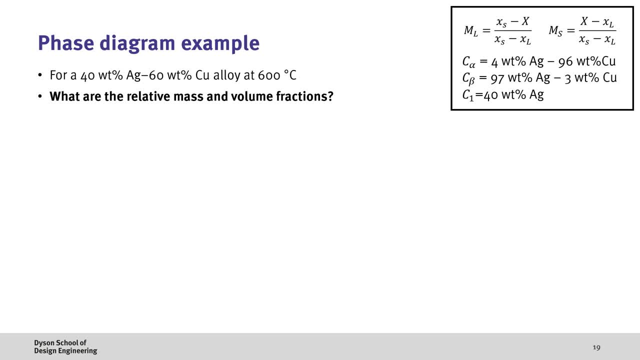 Ok. so now that we know we have two phases and what the composition of each phase is, the only missing element is now calculating what are the mass and volume fractions of each of these phases. To do this, let's first introduce a few definitions. 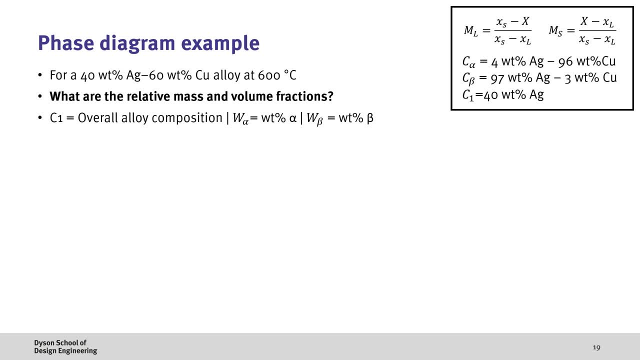 C1 is the overall alloy composition, W alpha is the mass fraction of alpha and W beta is the mass fraction of beta. We can then use the lever rule equation to calculate the relative amounts of alpha and beta, which are 61% and 39% respectively. 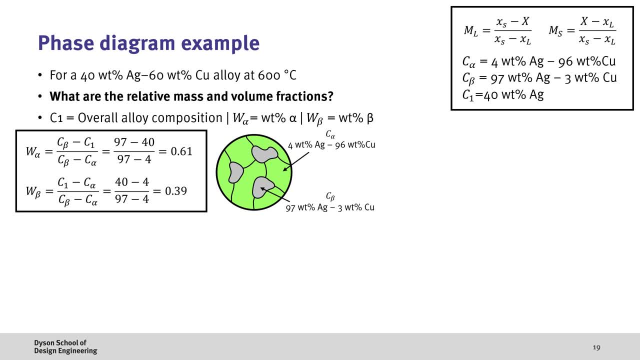 This looks slightly different to our earlier implementation. however, it's actually the same, since we just replaced liquid and solid with alpha and beta. Great, So now we know. So now we know the mass fractions. The final step in the calculations is to find the volume fractions. 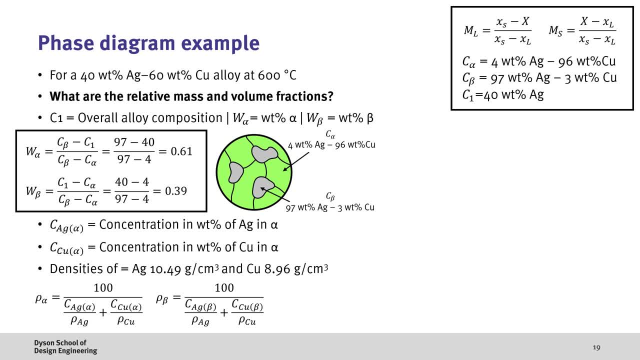 This requires us to revisit the amount of each element in each phase and to take an average of their densities. Here we define C Ag alpha as the concentration of silver in alpha and C Cu alpha as the concentration of copper in alpha. The density of silver is taken as 10.49 grams per centimetre cubed and the density of copper. 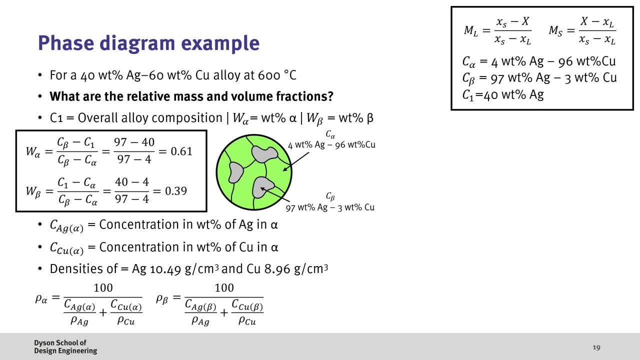 is 8.96 grams per centimetre cubed. Since we know the concentrations of each component and their densities, now we can calculate the overall density of each phase by using the equation below. If we then put the numbers into the equation, we can see that the density of alpha is 9.01. 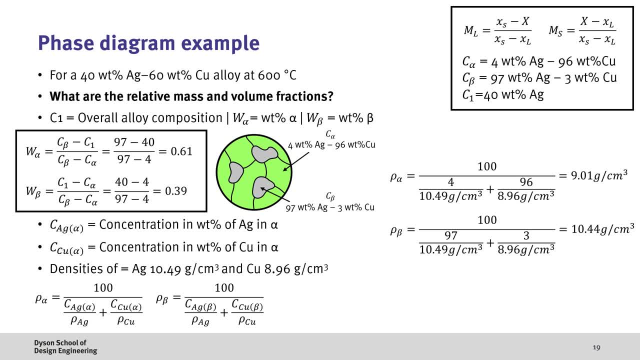 grams per centimetre cubed and that of beta is 10.44 grams per centimetre cubed. This makes sense, since alpha is copper rich, which has a lower density than copper. So we can calculate the overall density of each phase by using the equation below: If we then put the numbers into the equation below, we can see that the density of copper is 10.43 grams per centimetre cubed and that of beta is 10.44 grams per centimetre cubed. This makes sense, since alpha is copper rich, which has a lower density than silver, and 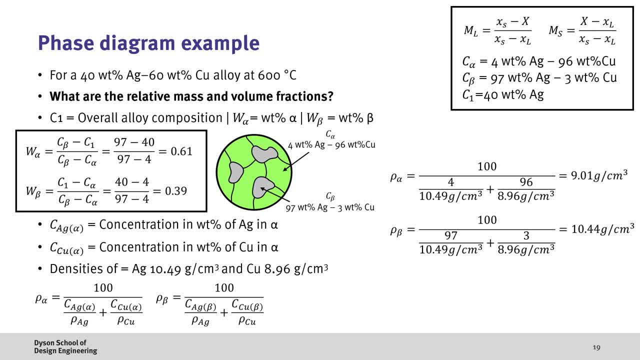 beta has more silver in it. Also, it's worth doing a quick check to see if the resulting densities are between that of the two base metals. Finally, now that we have the densities and mass fractions, we can calculate the volume of each component. If we take the ratio of the volume of a single phase and the combined volume. this then gives: 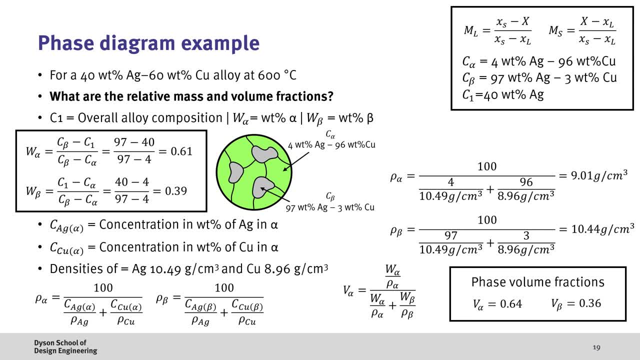 us the volume fraction of each phase, which are 0.64 and 0.34 grams per centimetre cubed. This gives us the volume fraction of each phase, which are 0.64 and 0.34 grams per centimetre cubed. This gives us the volume fraction of each phase, which are 0.34 and 0.34 grams per centimetre cubed. This gives us the volume fraction of each phase, which are 0.34 and 0.34 grams per centimetre. 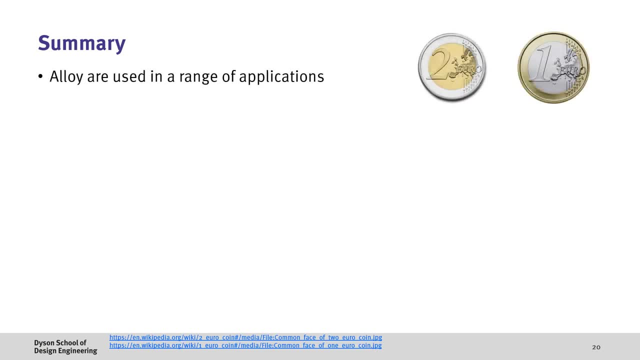 cubed. This gives us the volume fraction of each phase, which are 0.34 and 0.34 grams per centimetre cubed. So to summarise, hopefully you've seen that alloys are used in a range of applications, but changing their composition can drastically change their physical and chemical properties.